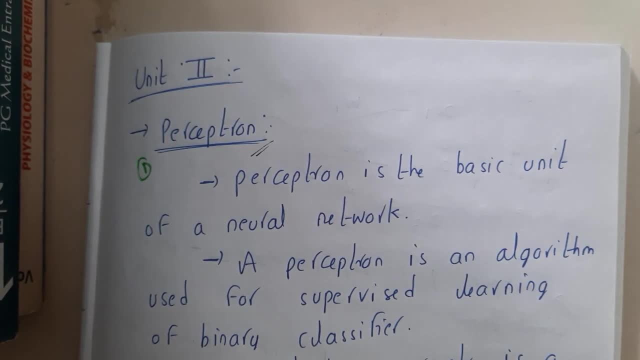 they'll be saying that for image processing and all those things, neural networks will be used- convolutional neural networks, Any neural networks names. they'll be saying: guys, even I don't know those names, Okay, yes, So they'll be saying multiple names. So we'll be getting scared like what are these all things? Okay, and 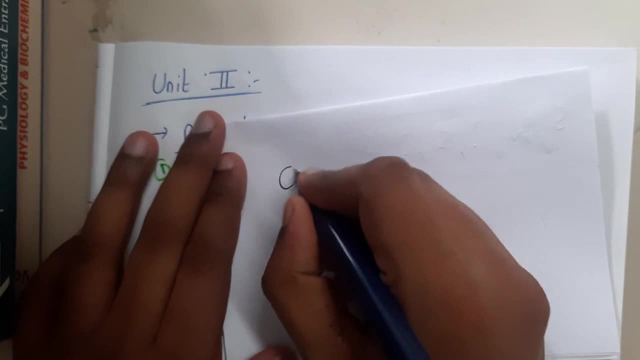 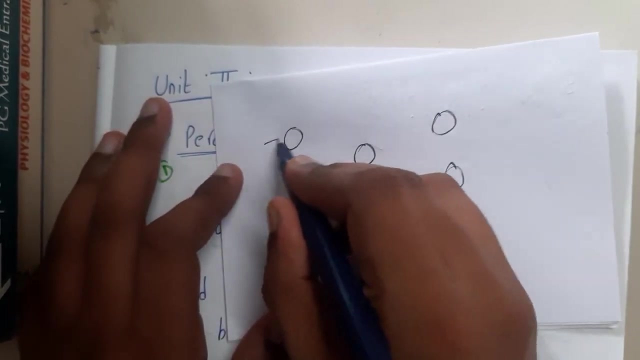 whenever, if you ask some faculty or someone, they'll be just drawing this diagram for neural network. So they'll be saying these are inputs Okay. so these are inputs Okay. so you'll be giving some inputs here, Okay. and these are all connected with all combinations, guys, Okay, okay. 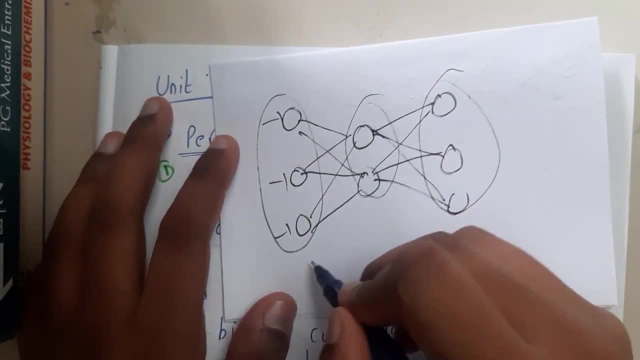 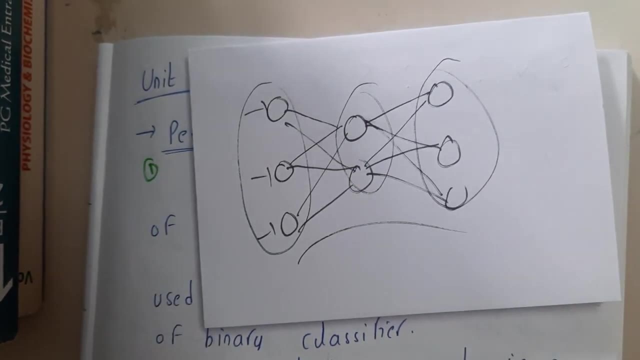 Okay, and this is your input layer, this is the output layer, this is the hidden layer. So this is a simple concept which they teach and it looks really easy, right? Yes, but we don't understand. we don't know exactly how this works, Like, what is the behind the math? for all those, 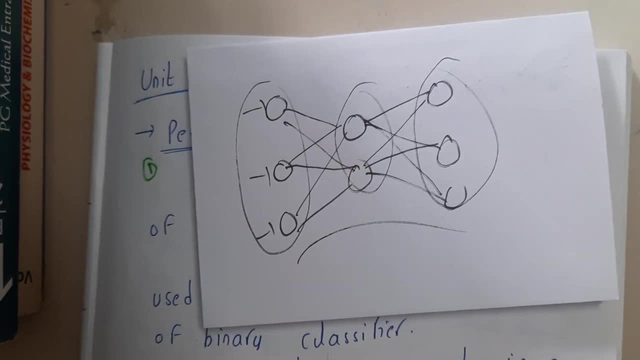 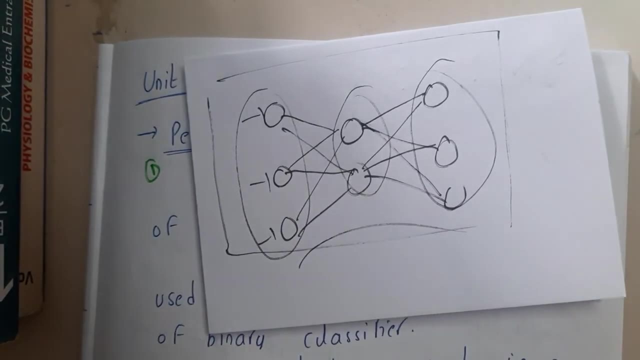 things right. So we'll be having these kind of doubts, but these are really interesting, as if you ask me right? Yes, So basically let us start. So this is a neural network, guys. Okay, in total you can call it as a neural network. Okay, so a smallest component or a cell of a? 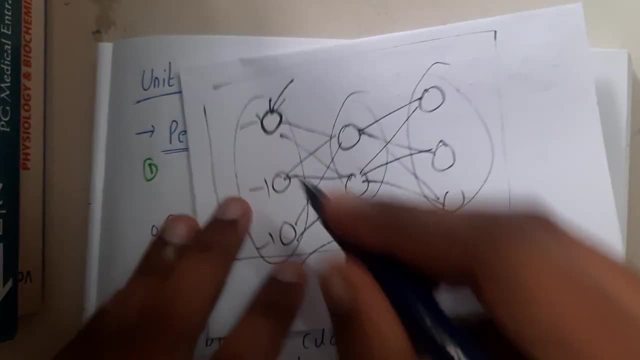 neural network. don't call it cell. the name of it is called as perceptron guys. So this single bubble, you can call it as a perceptron guys. So this is a single bubble, you can call it as a perceptron guys. 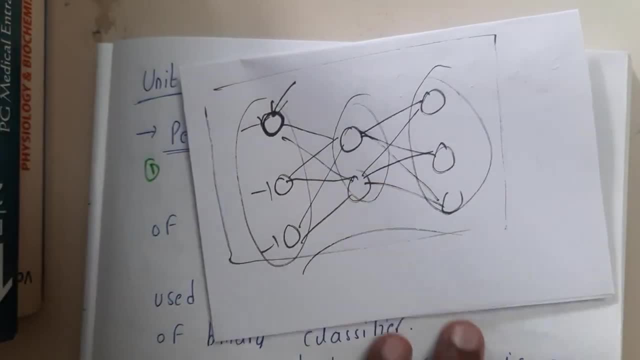 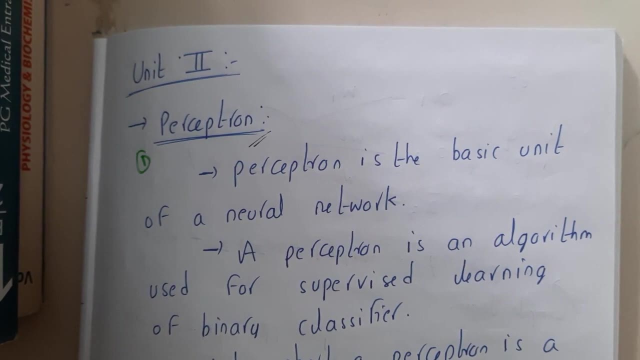 Okay, so it is the smallest unit in a neural network. Okay, so perceptron is the basic unit of a neural network. Okay, so I hope everyone got a clear idea right. So what is perceptron? first of all, because it's really important to understand this. That's the reason why I'm 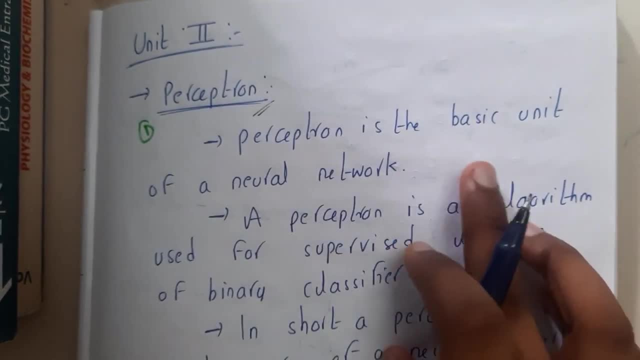 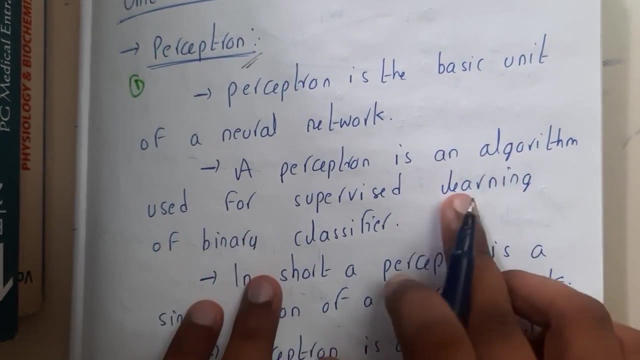 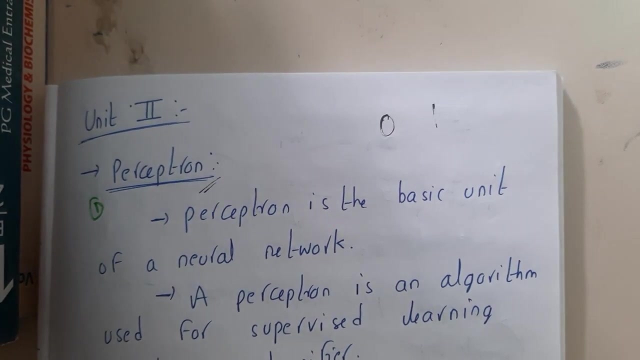 stressing on it. Okay, yes, let us continue. So perceptron is a basic unit of neural network A perceptron is an algorithm used for supervised learning of a binary classification. Okay, so to classify two things. it might be zero, one pattern. you can say in simple words: because perceptron 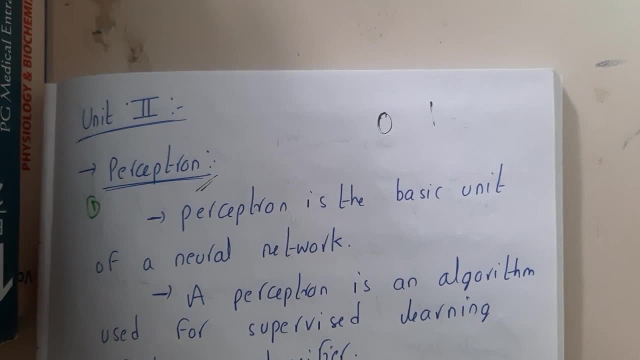 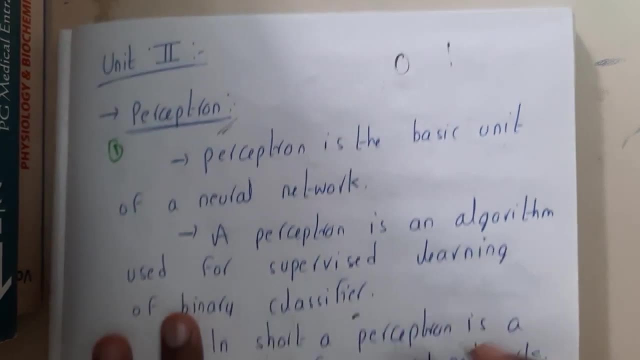 cannot be used on complex things, Okay, and it cannot work even on some easy things also. So there are some many drawbacks. you can say in perceptron, like anything cannot solve each and everything, right, guys? So in that way, okay, yes, So it is best among itself. Okay, yes. So in short, 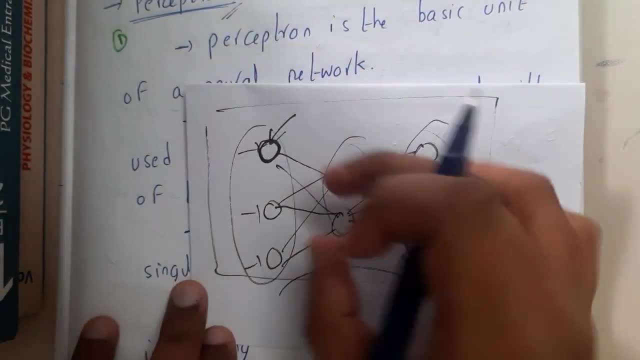 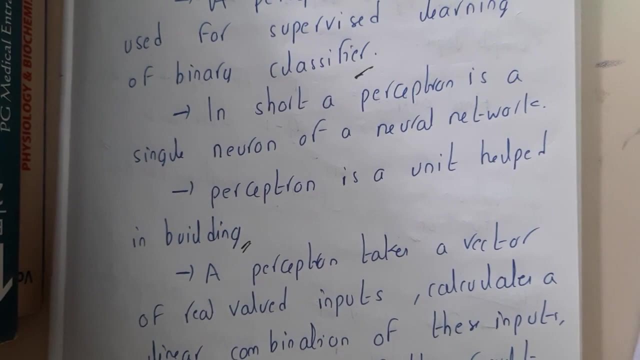 a perceptron is a single neuron of a neural network, So basically among a whole neural network, a single neuron is called as perceptron. Okay, so perceptron is a unit which helps building of a neural network. So basically combining these perceptrons only. 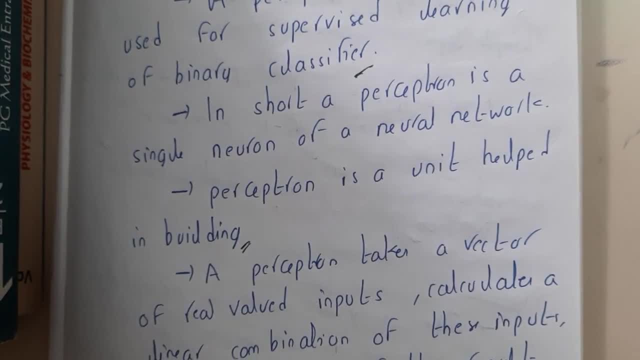 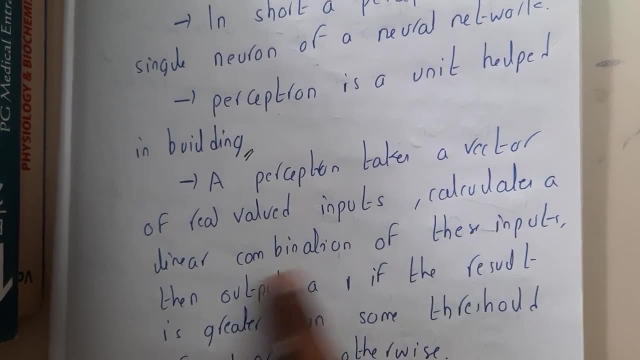 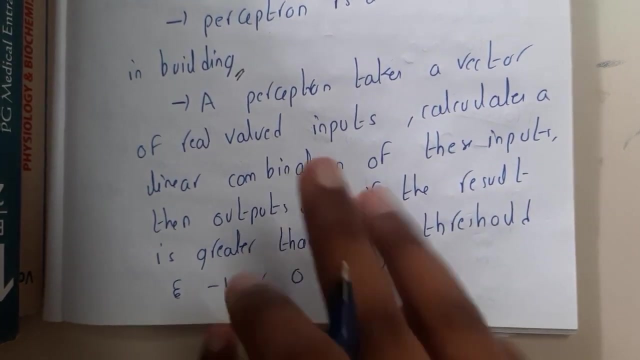 we are forming a neural network, guys, right, Yes, Okay. so a perceptron takes a vector of a real value input, calculates a linear combination of these inputs, then outputs of one if the result is a greater than some threshold and minus one otherwise. guys, don't get scared with these kind. 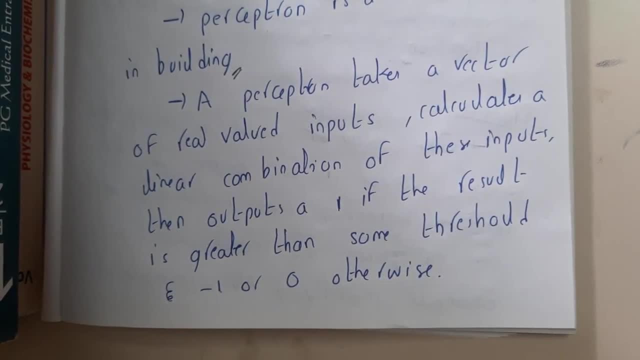 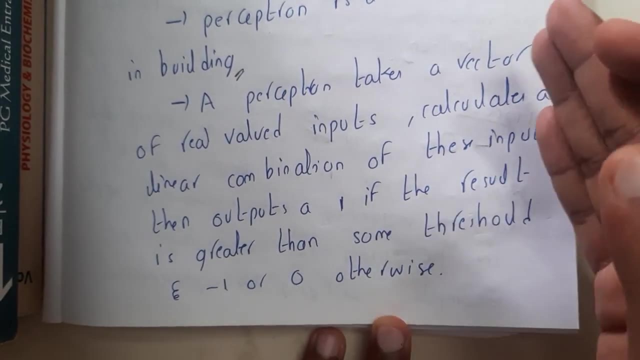 of theoretical parts, guys, because I'll be taking an example And I'll be making it easy for you, Don't worry. Okay, Yes, So we will be having some math function. you can say So. based on that math function one, it will give some if it is greater than some threshold. you'll be getting one as the 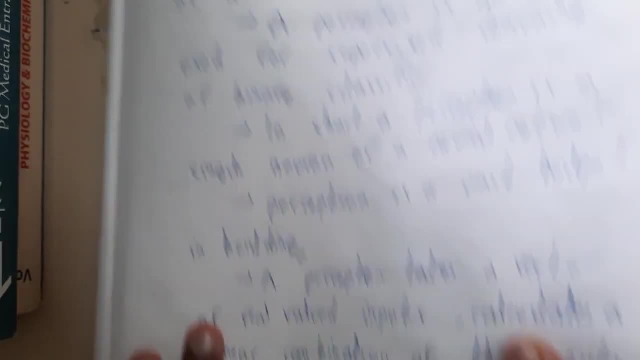 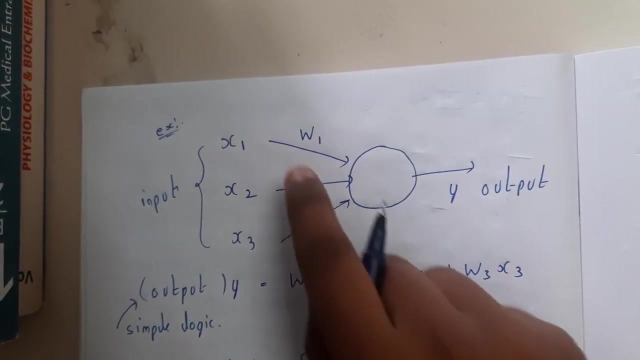 result: If it is not greater, you will be getting minus one or zero, based on your method, which we have selected. Okay, Yes, So firstly, let us draw a small diagram of a perceptron. Okay, So, basically, this is our perceptron, guys. So it is having multiple inputs, right? So this x one indicates: 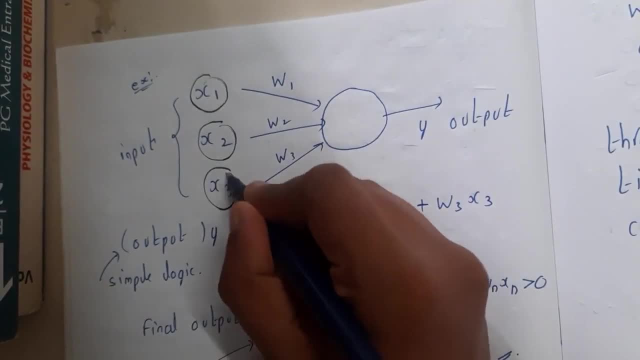 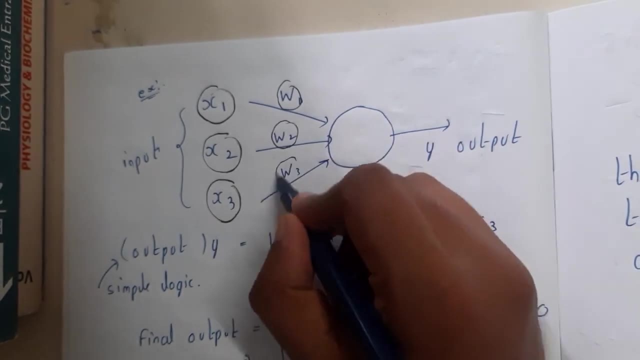 input one x two indicates input. two x three indicates input three. Okay, And w one inputs indicates a weight of that path, w two indicates weight of the second path, weight of the third path, And at the end you will be getting an output. Got it? Yes, So this is a simple, simple. 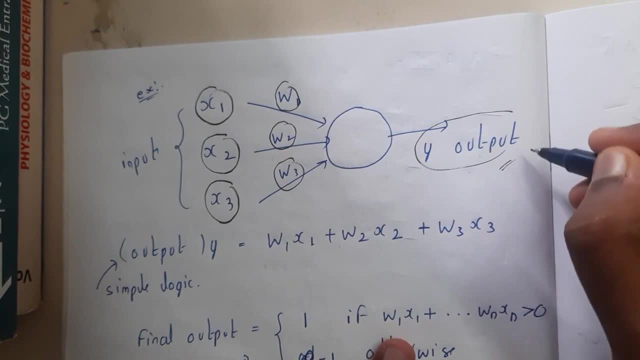 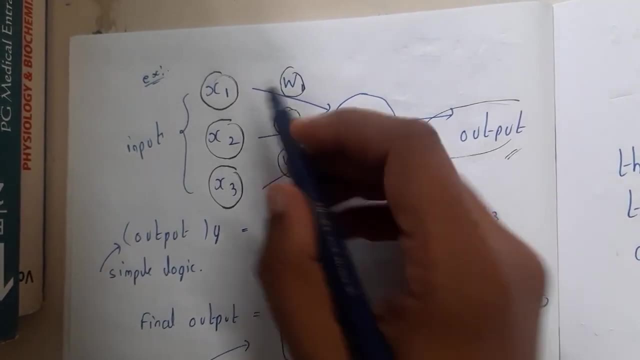 diagram, you can say, Okay, So basically you'll be saying that, okay, so we'll be getting some output. So is there any relation between the input and output? Yes, there's a relation. So the relation is nothing, but y is equals to x. one into w one plus x two into w. two plus x three into w. 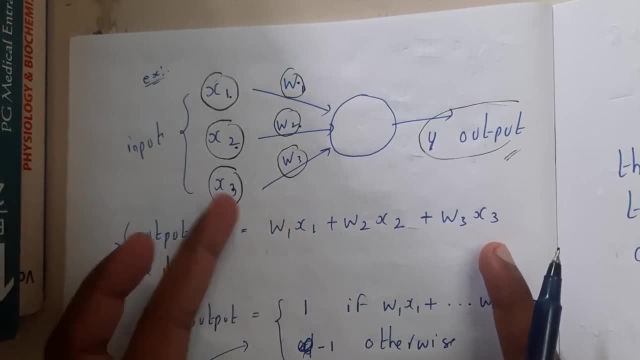 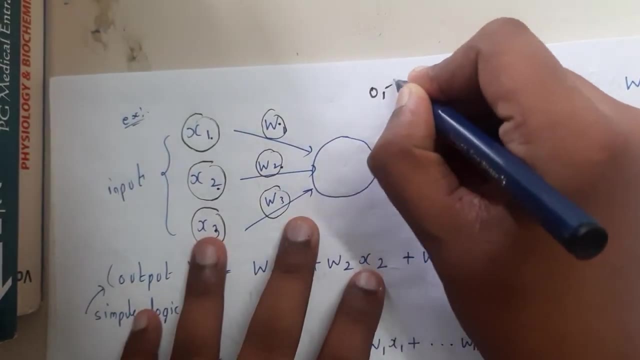 three. Okay, So this is a simple math, guys. I think everyone can write it right. Yes, And the main equation I told you right? So it should be zero or minus one or plus one, right? So I gave you these two options. So if it is greater than some, 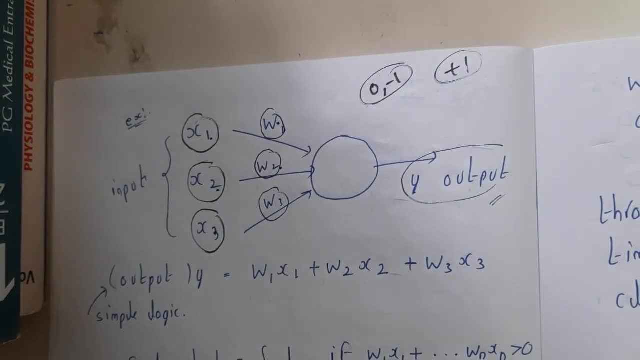 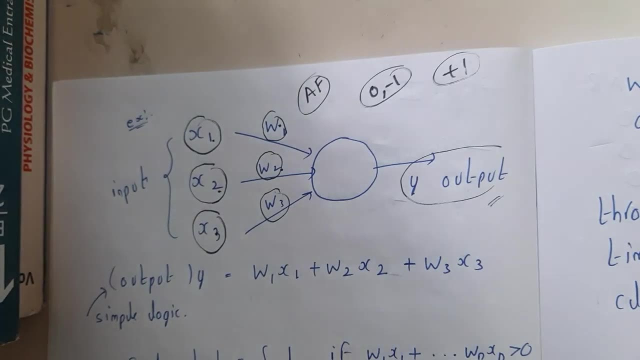 threshold it will be plus one, else it will be zero or minus one. So I told you that right? So that function, or that math equation, is called as activation function, guys. So whenever you try to read from any textbook or anywhere, they will be saying that it should be greater than. 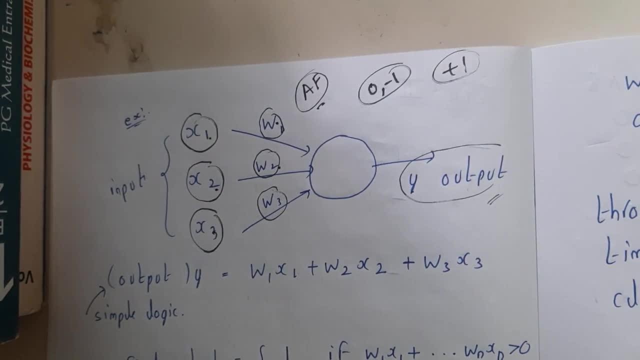 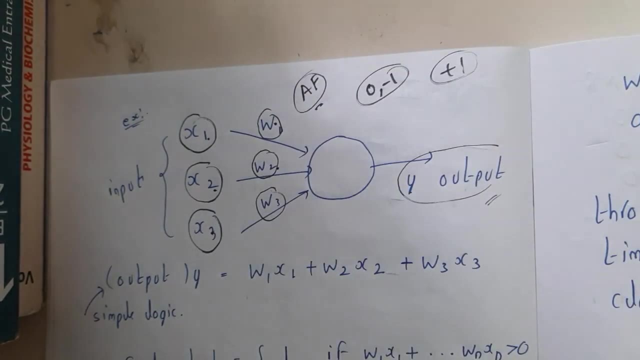 activation function, but they never try to explain you clearly what is activation function, guys? So the activation function is the one which decides whether you are going to get the result: the one, or it might be zero or minus one. So that is the main function. you can say So, basically. 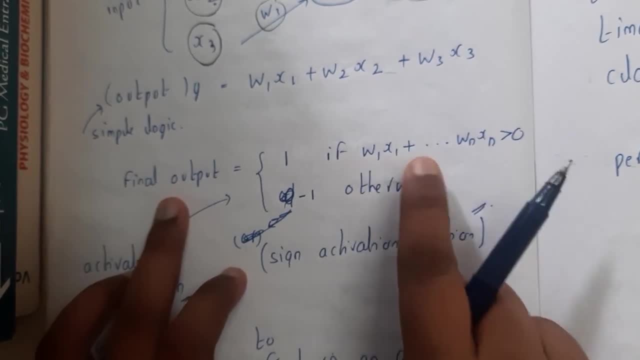 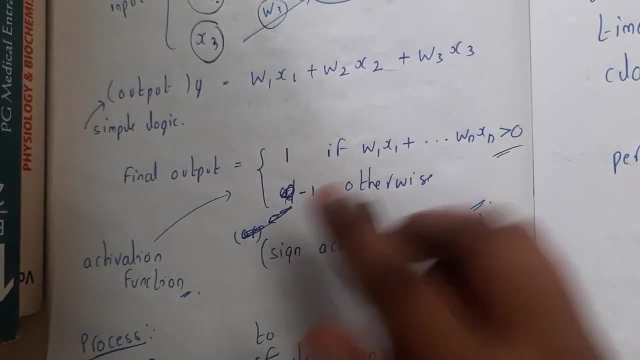 it might look in this way: So one if w one x one plus w two x two, and so on, up to w and x n is greater than one. So if the sum is greater than one we will give one, else we give minus one. So 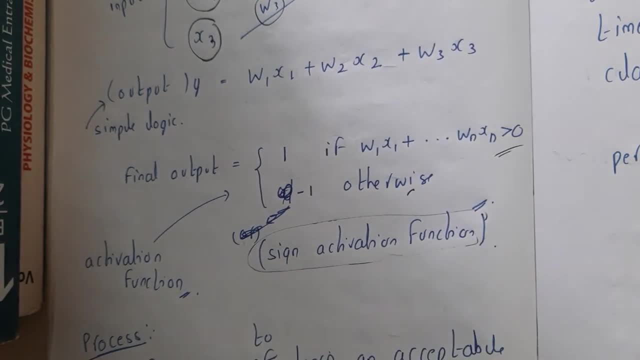 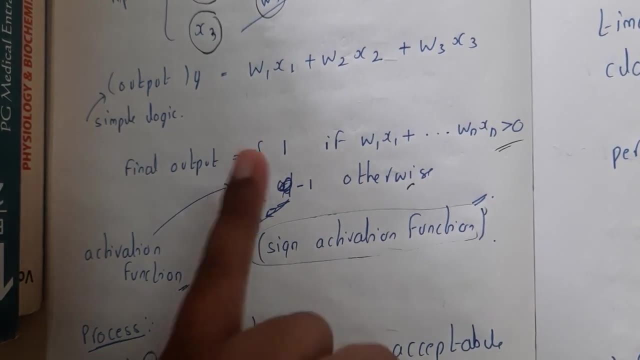 in this way. so this name of this function is nothing but sign activation function, guys, Okay, Yes, So this is nothing but the activation function. So I hope everyone got some basic idea about the terminologies, right? So what is a neuron? What is an input? What is a weight? What? 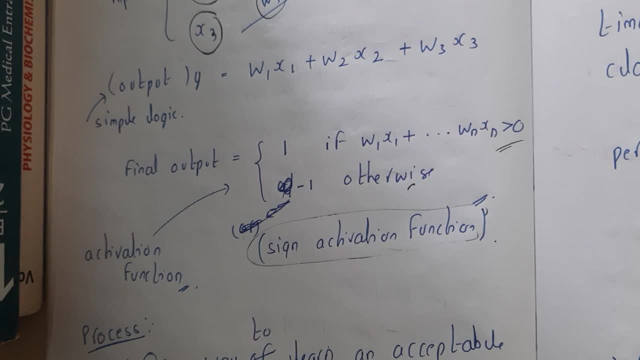 is the activation function, All those things right, Yes, So these things could be asked for one or two months, And if you write in your resume that you are interested in machine learning and if you did some projects, you should know all these definitions, guys, because at any moment of 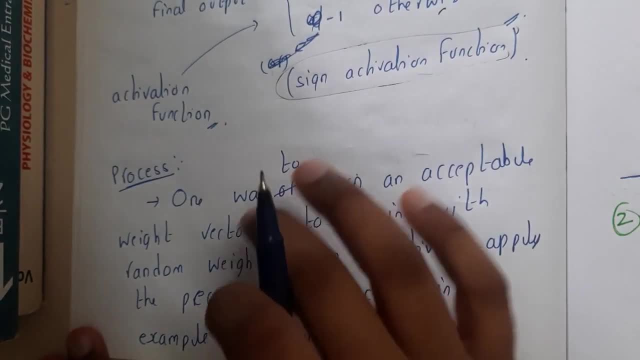 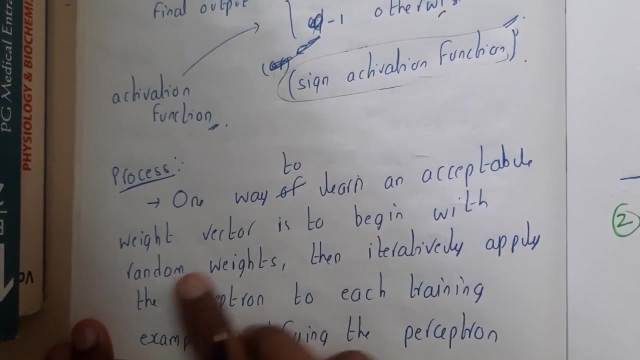 time in interviews they might ask you: right, Yes, So let us continue. So what is the exact process? it is going on. Okay, So let us go through it. So one way to learn an acceptable weight vector is to being with random weights. So basically, you might be asking me: so why this? 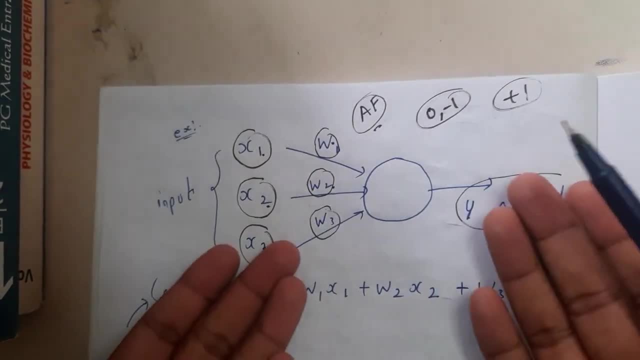 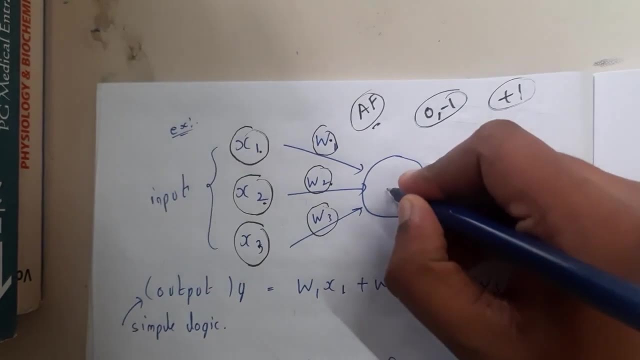 process came now. So basically assume that there should be some relation, right? So why are you building this neuron? Okay, So you might be saying that, okay, so I want to perform some operation. So I hope everyone knows and operation: right, A and D, That is on basis of input 0, 0, it will. 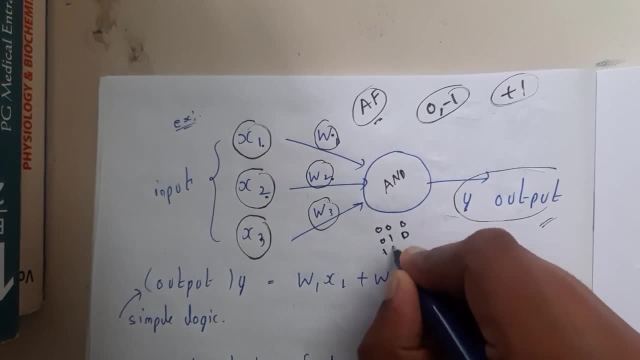 give 0.. On input of 0, 1, it gives 0.. On input of 1, 0, it gives 0.. On input of 1, 1, it gives 1.. So only in this situation it gives 1.. So I want to build a perceptron for this equation. 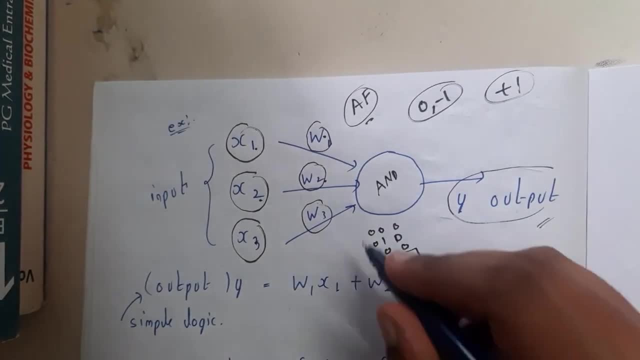 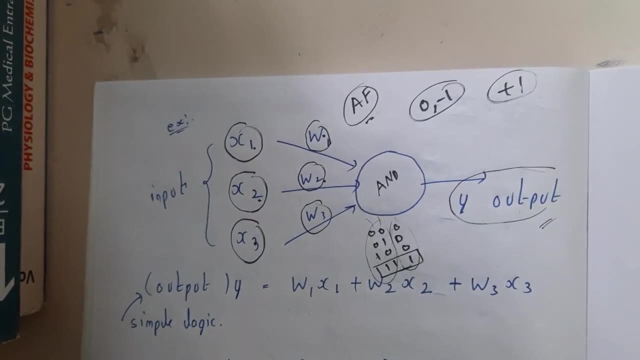 Okay, So if I want to build this initially, I know the inputs- Once it will be 0 or this, So I expect this output. right, So by giving this inputs, I expect this output. So, basically, to build this, I should logically find the values of: 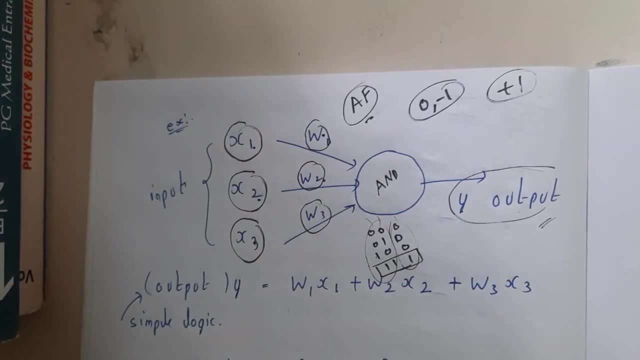 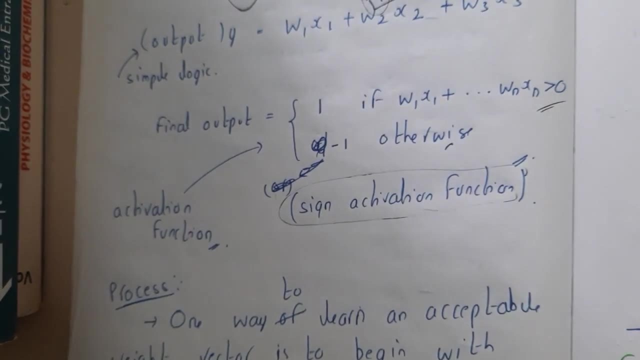 these things, right? Yes, So your question will be okay. so, are there any fixed values? Your question will be right, Yes. Yes, The answer for it is no. We are not having any fixed values, guys, Okay. Sometimes in examination they will give these weights, guys Okay. 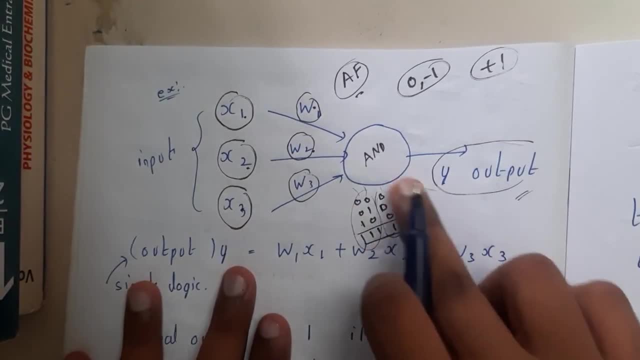 And they will say as to adjust them so that it satisfies the R equation. So basically, they will say: here the weight is 1.2.. Here the weight is 0.6.. Okay, And they will say that it should follow this condition. 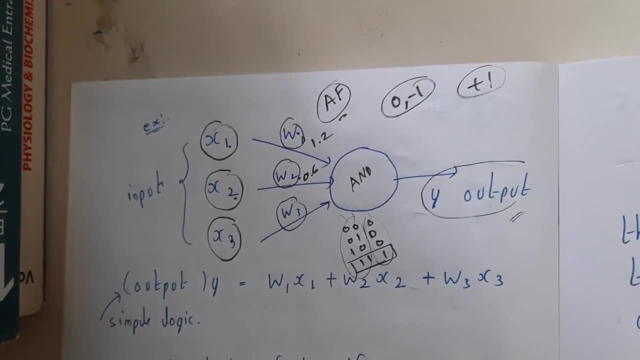 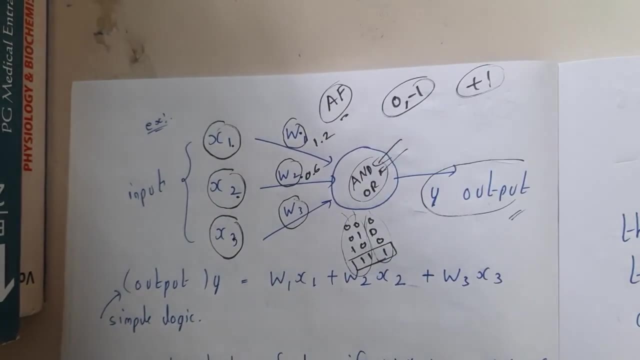 update the weight somehow. So that is the thing they will say and they will give you right. Yes, So these are most commonly asked So for. and and or they will ask guys commonly. So these two examples we will be discussing in the next two lectures. Okay, Yes, So let 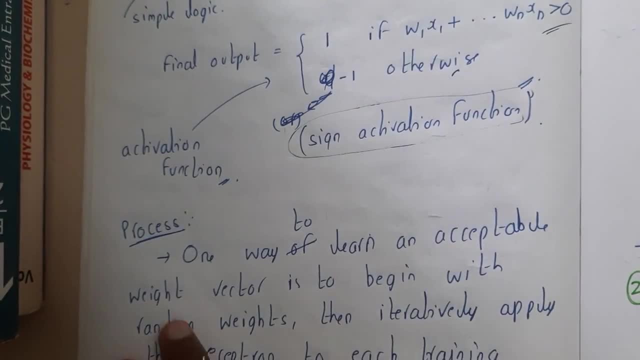 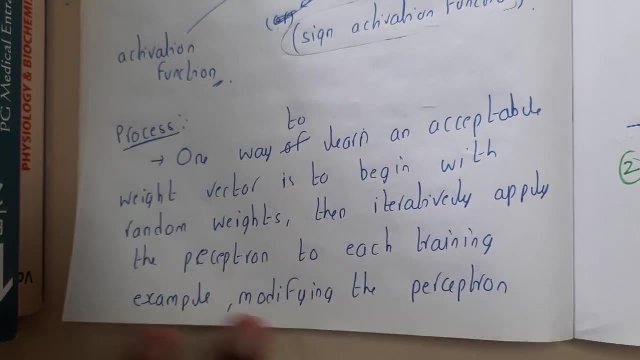 us go through the process now. Okay, So one way to learn an acceptable weight vector is to being with random weights. The iterations apply the perceptron to each training example and modify the perceptron with the weights which are misclassified. Okay, So I know. 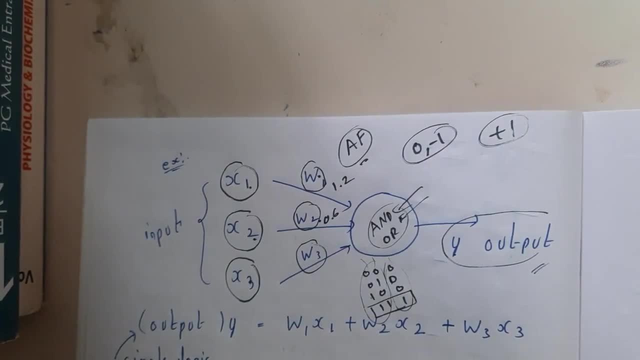 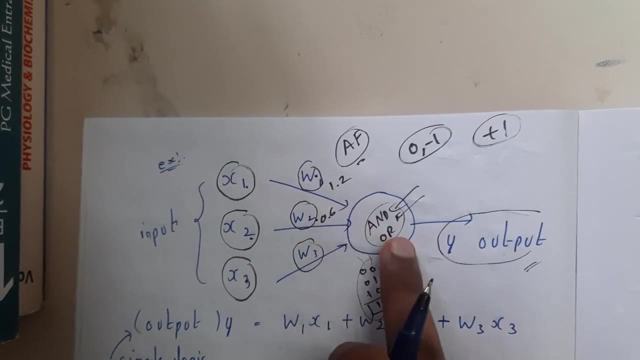 that most of you did not get what it is trying to say. So basically, initially we will be giving these unassumed or assumed weights, right? Yes, So with this assumed weights you will be entering inside. Okay, So once we enter inside you will be getting an output. 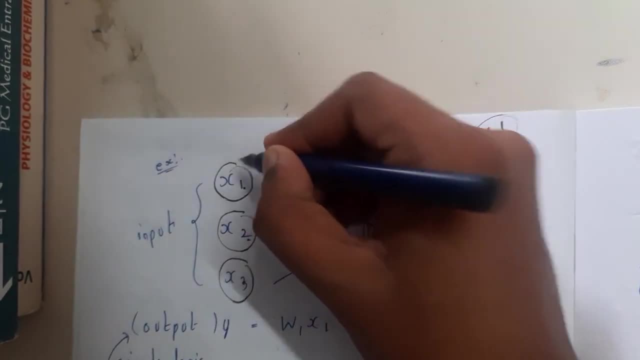 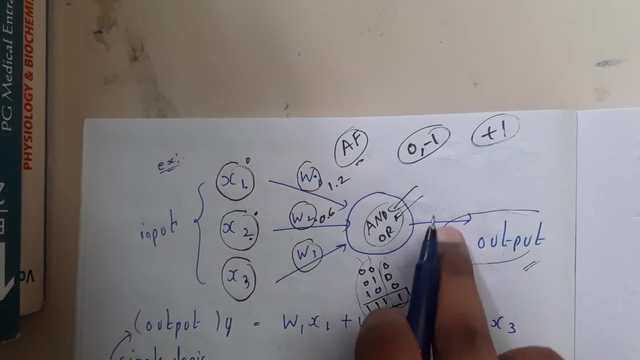 right, So with this input, So basically these are the inputs. So let me do it only now, only to make you late, right? Yes, So 0 into 1.2 is 0.. 0 into 0.6 is 0.. So at the end we got. 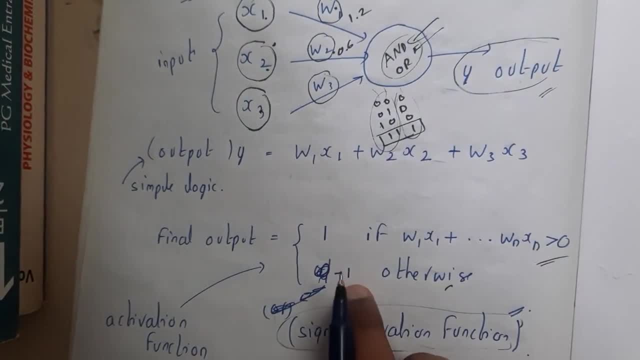 the result as 0.. So, based on our function, if it is greater than 0,, so assume that it is greater than 0. This is otherwise 0.. Okay, So in that situation we got this result. Similarly, when you try: 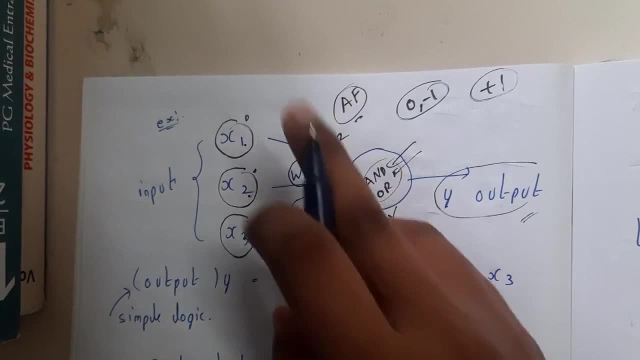 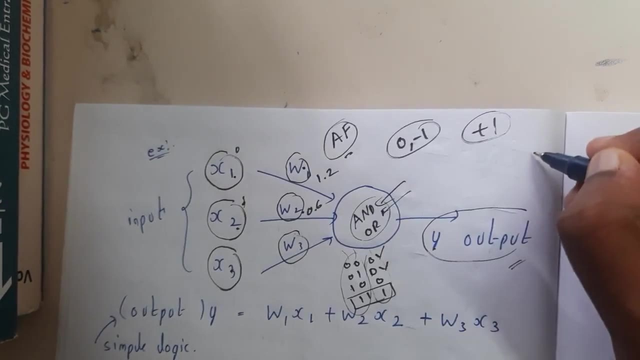 this again, you will be getting 0 only. So, basically, 0 into 1.2 is 0.. 1 into 0.6 is 0.6.. Here we got 0.6, right, So our condition here? let us assume in this way, guys. So. 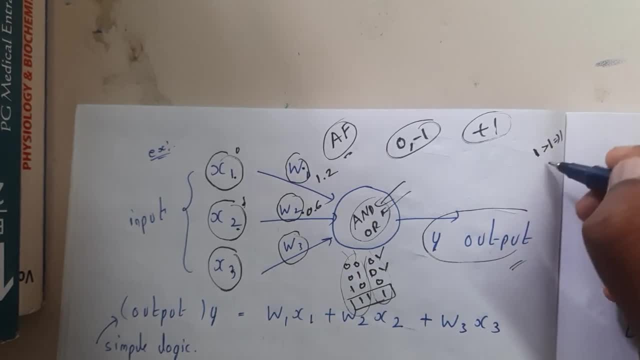 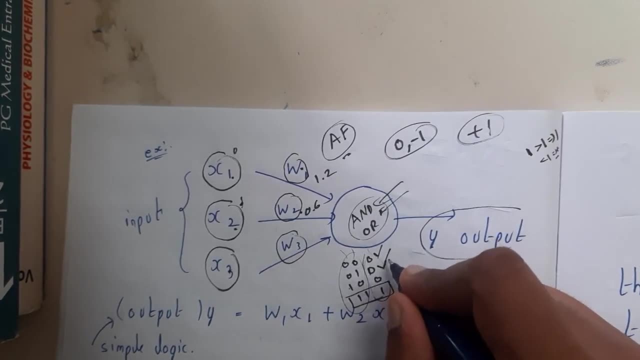 if it is 1 or greater than 1, you will result 1.. If it is less than 1, you will say as 0. Logic: Okay. So as it is less than 0, less than 1, I will be taking 0. Okay, So similarly, 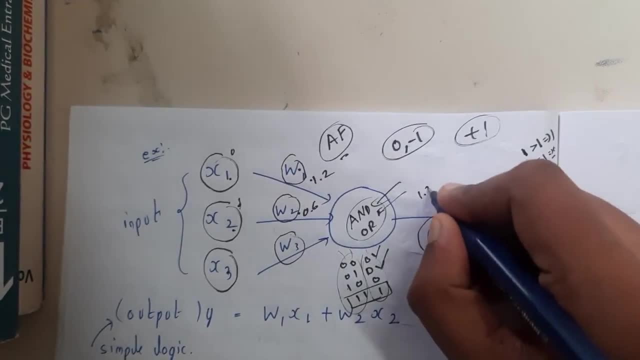 the next time. So if you take this 1, we will be directly getting 1.2 here. So which is greater than 1, we should give 1, but the answer is 0. So, basically, you need to adjust this somehow. 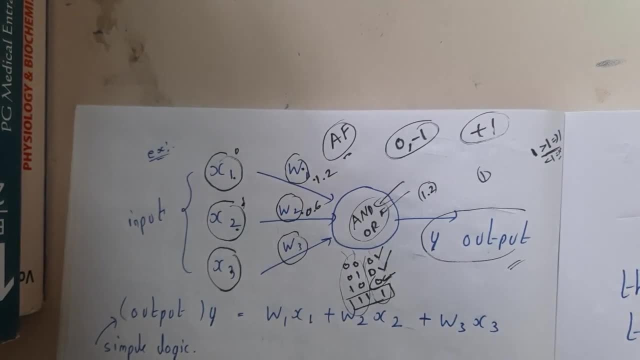 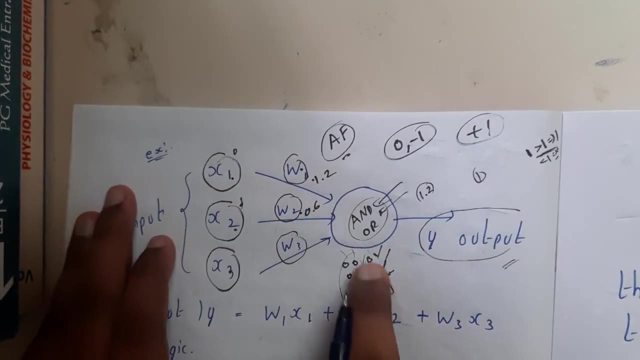 right. So, using backtracking, we will adjust guys. Guys, I will be discussing about this in detail in the next lecture, So do not think too much. Okay, So I just gave you an overview like how you are going to do. So you will be calculating them and you will be checking. 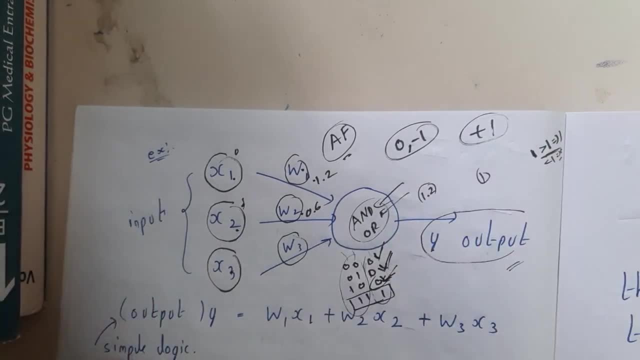 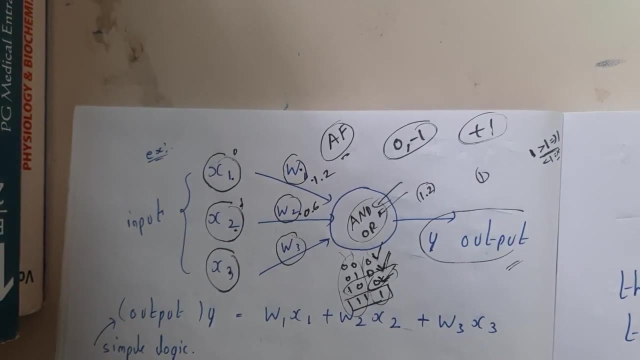 you will be matching your answer, your expected output. So if it is matched, it is 100% okay. If it is not matched, you will modify the weights. Simple logic, right? So your question will be okay. you are saying: modify weights, modify weights. Then how are we going to do?